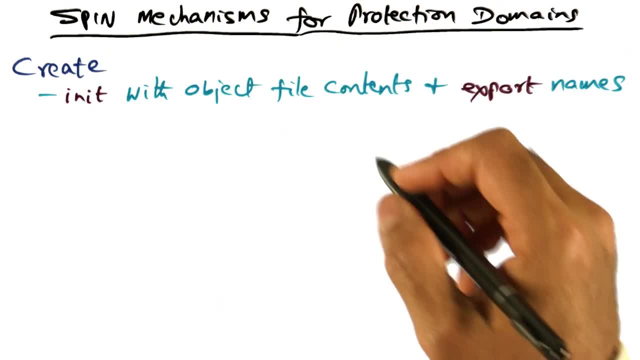 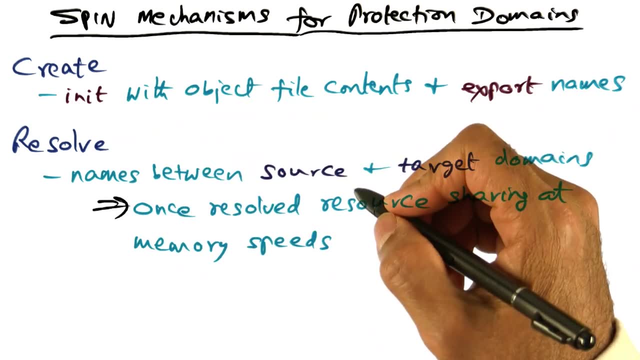 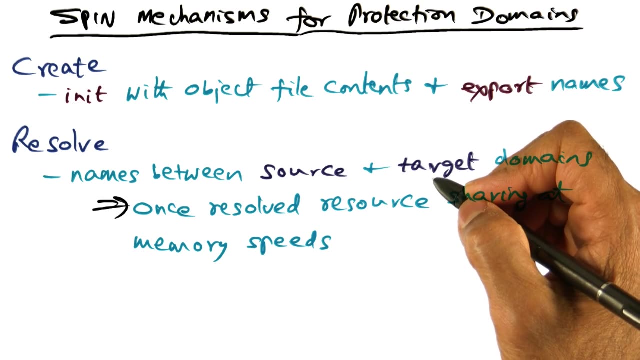 export the names using this create mechanism that's available in SPIN. The second mechanism in SPIN is resolving names. If one protection domain wants to use the names that is there in another protection domain, the way it can accomplish that is by using this resolve primitive that's available in SPIN. 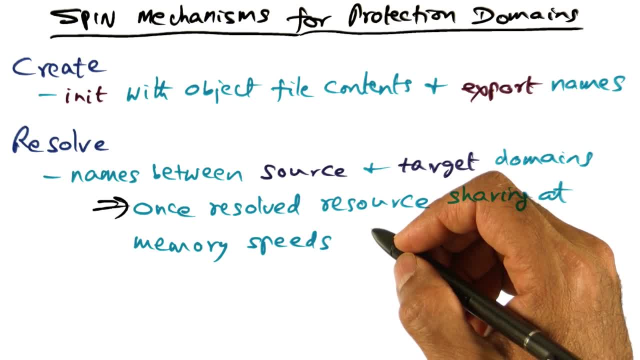 Resolve is very similar to linking two separately compiled files together. that a compiler does routinely. So you may be very familiar with the compilation process, where you may separately compile files and once you have done the separate compilation of the files, then you go through a link phase of the 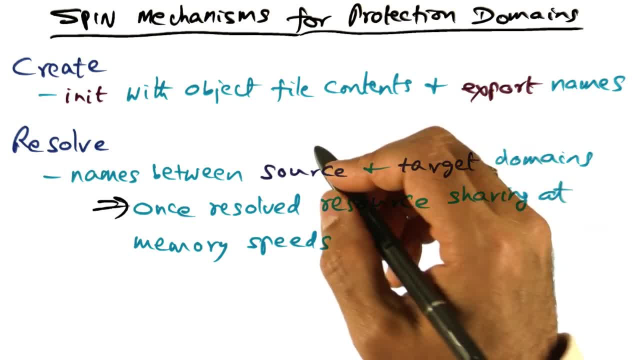 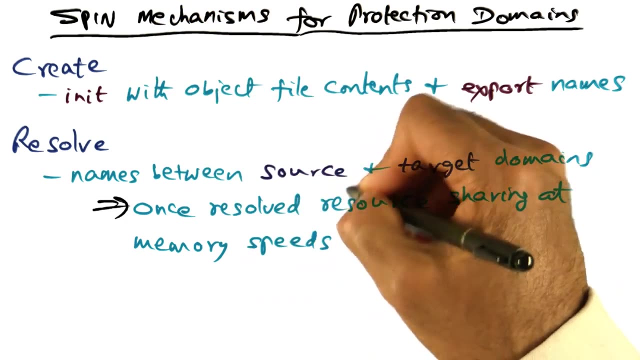 compiler, where the linker resolves the names that are being used by one object file with the names that are defined in another object file. That's the same thing that the resolve mechanism of SPIN does, is it resolves the names that are being used in source, which is a logical protection domain, and the target. 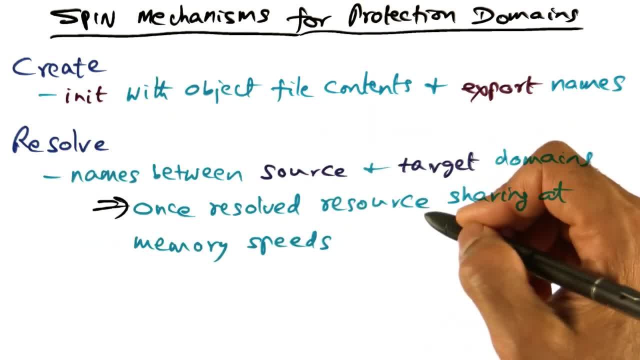 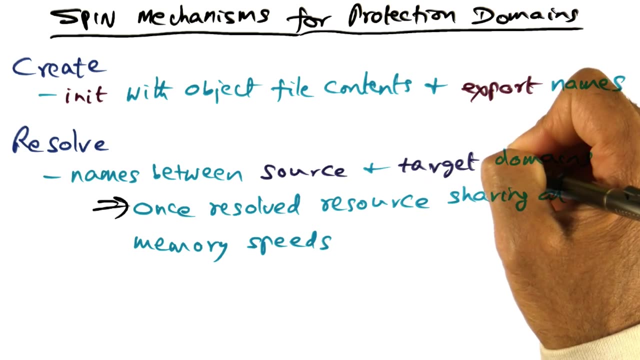 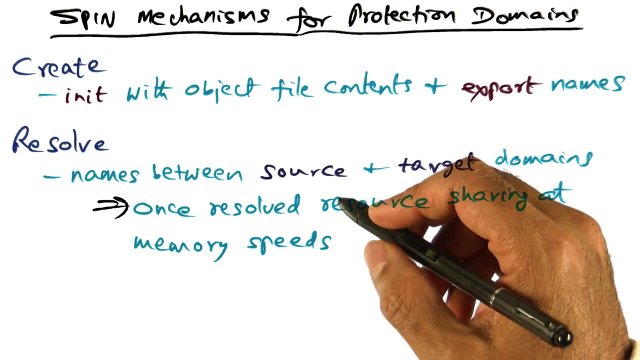 which is another logical protection domain. as a result of this resolve step, The source logical protection domain and the target logical protection domain are dynamically linked or bound together, And, once bound together, accessing methods that are inside this target protection domain happens at memory speeds, meaning it is as efficient as a 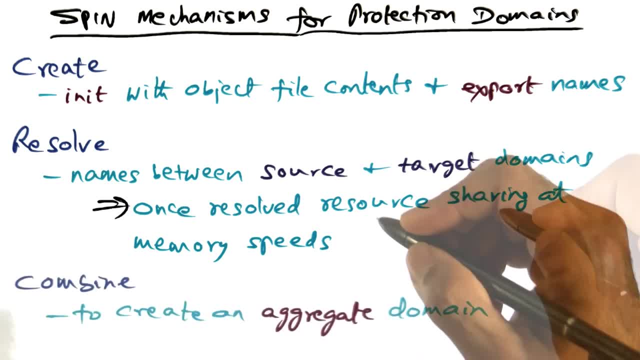 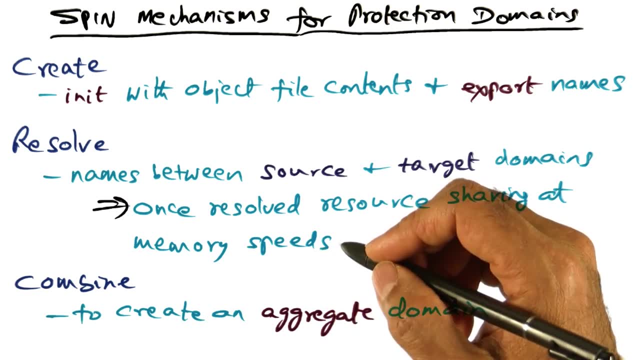 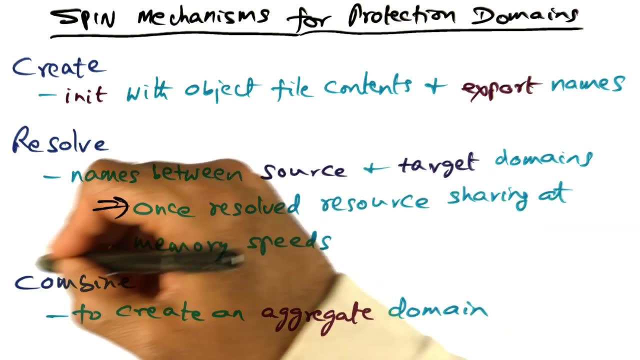 procedure call once this resolve step has happened. As I mentioned before, to reduce the proliferation of small logical protection domains, you may want to combine protection domains to create an aggregate, larger protection domain, And SPIN provides a mechanism for that, which is the 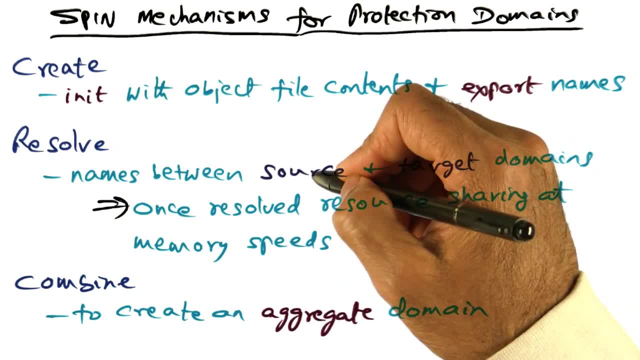 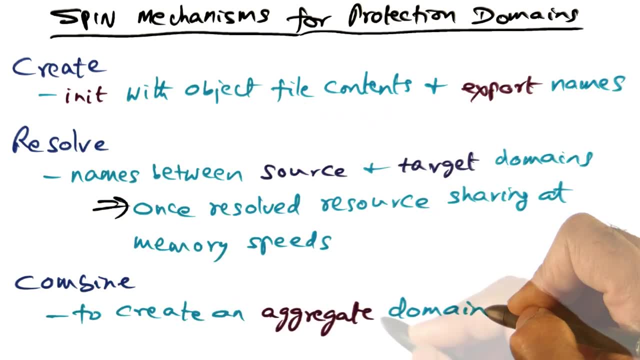 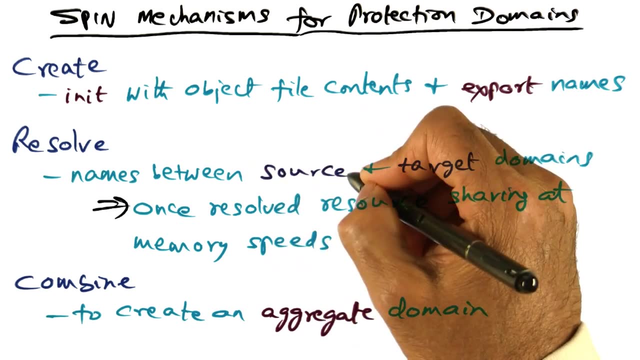 combined mechanism. Once the names in a source and target logical protection domain have been resolved, they can be combined to create an aggregate domain And the aggregate logical protection domain will have entry points, which is the union of the entry points that were exported as names.